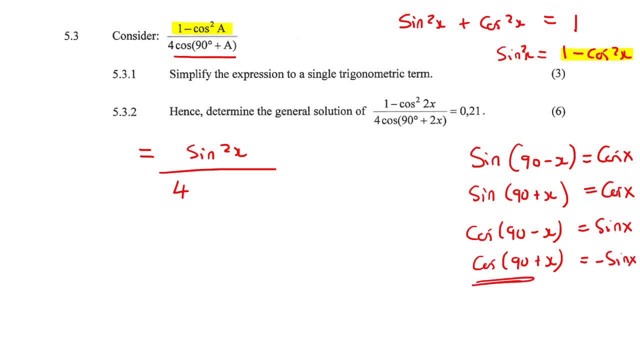 weird one. This one becomes negative sin squared x. This cos squared 90 plus that one becomes negative, And that's actually the one that they gave us here, the sneaky people. So what we need to do is change this into negative sin squared x, because 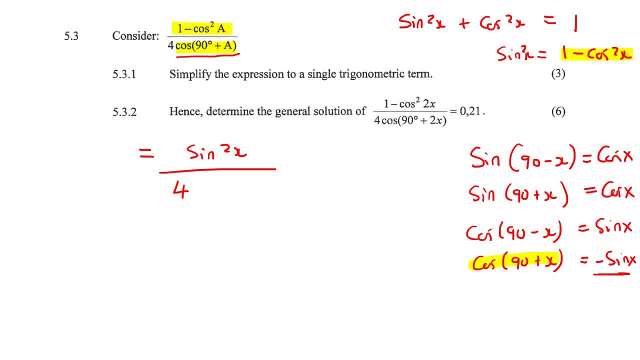 you see, we have it there and we have it there, Okay, So we're going to change it to negative sin x, like that, And so we end up having sin squared x over negative 4 sin x, And so what happens now is that you can cancel. 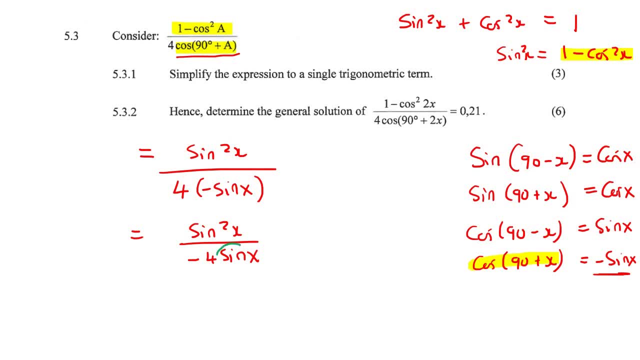 out one of these sins. Okay, So you can cancel out this sin over here with one of the sins at the top, And so we would end up having one sin x left over at the top and then at the bottom. you're just going to end up having negative sin x, And so. 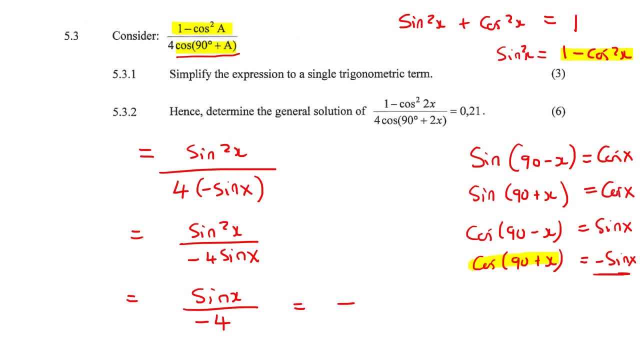 this is going to be 2 sin squared x. So if you want to write this in a better way, you can just say negative sin x. You could say negative, you can just put the negative in the front, So negative sin x over 4.. You could also write it as negative: 1 quarter sin x. 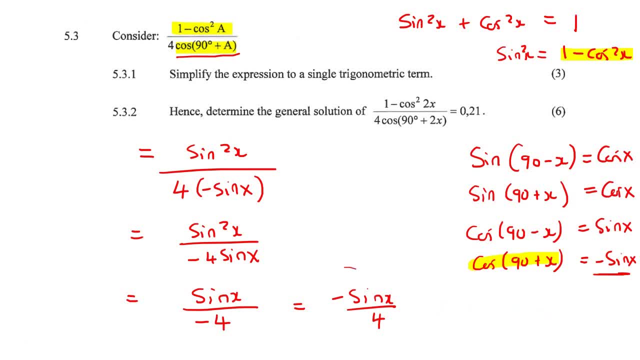 if you wanted to, Okay, But I think what I'm going to do is I'm just going to leave it like that. Okay, And I realised that all throughout this video, I've been using x instead of a. Please don't shoot me. I mean, that was just a small mistake. It's not that serious, Hey. 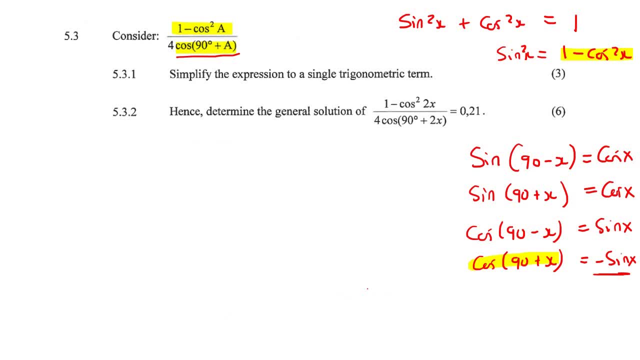 guys. Okay, so let's just write down our answer here. we said negative sin x over four. the next question says: hence determine the general solution of this. okay, so what you guys need to do is you need to try see the pattern between these two things, between this one and between that one. so let's have a look at. 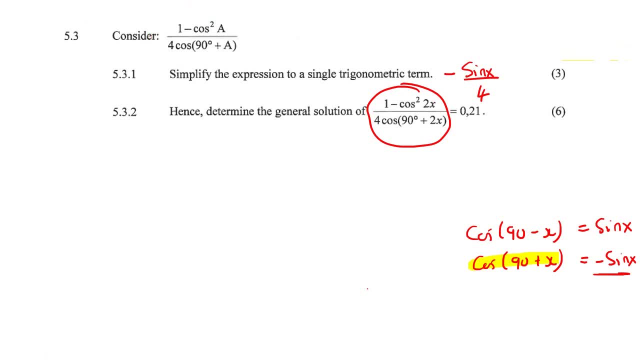 those carefully. so here they're using a and a, here they're just using a 2x and a 2x, but besides that everything is exactly the same, right? so we learned in the previous question that one minus cos squared a over four cos, 90 plus a. we learned in the previous question that that becomes minus. 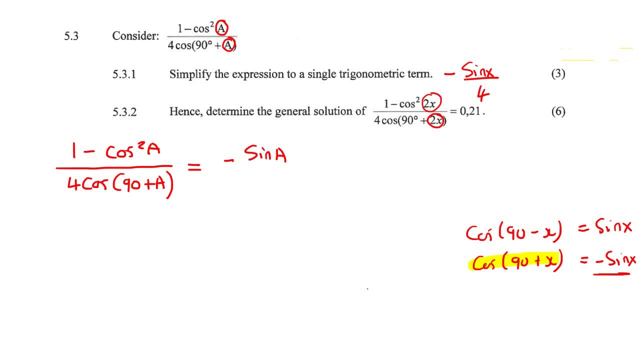 and now i'll change it to a sorry you, I did apologize, but I was using x's the whole time. We know that that turns into that. So then, what they want us to do is to think about what would this become then? Well, you can just follow what we did here. 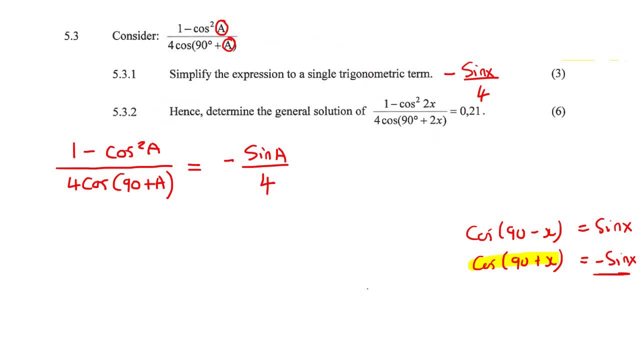 but you don't have to go do everything because they said hence so we're using the previous answer. So then we can say that 1 minus cos squared of 2x over 4 cos 90 plus 2x. We can then change that to minus sin. 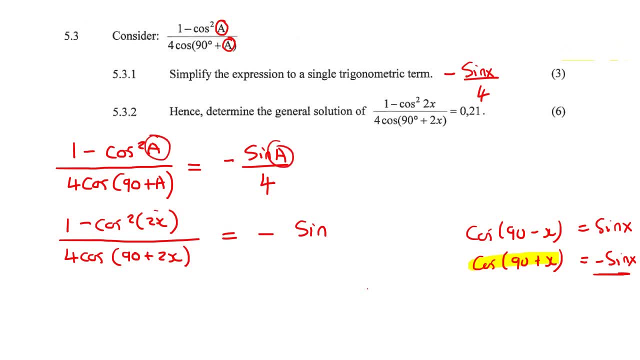 Now you just copy the angle. So if this was a and this one's a, now this one's 2x, So then this one also becomes 2x over 4.. Okay, so that's what we can change this part into. 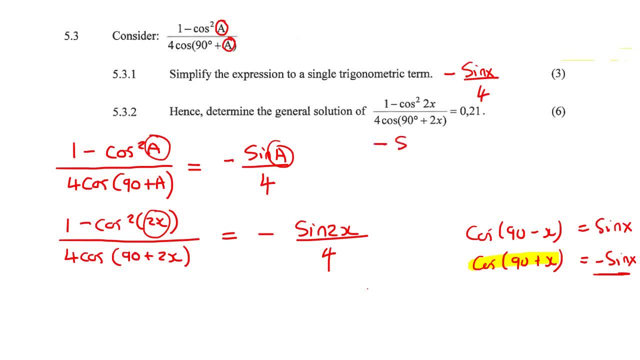 So we can rewrite this equation now, as minus sin 2x over 4 equals to 0 comma 2, 1.. And now this just becomes a whole brand new general solution question. So what we need to do is we need to try to get this sin 2x by itself. 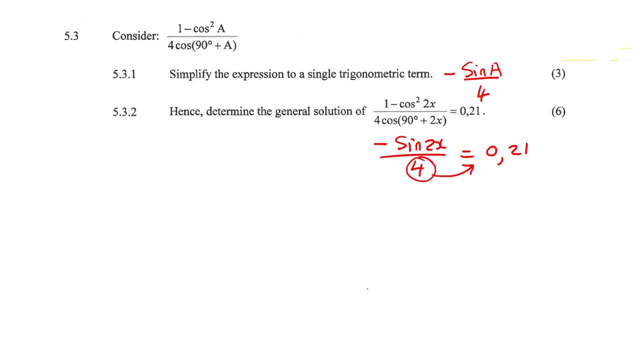 So what I would do: first I'll take this 4 and I'll multiply it across, So that's going to end up giving us negative. sin 2x equals to 0 comma 8, 4.. Okay, then this negative we can divide by that negative. 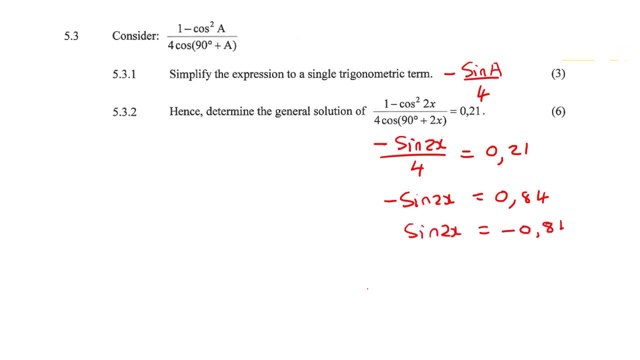 So it becomes: sin 2x equals to negative 0 comma 8, 4.. Okay, so I'm going to start over here now, or carry on over here. should I say Okay right now? this becomes a fairly basic question. So what we need to do now is get the reference angle. 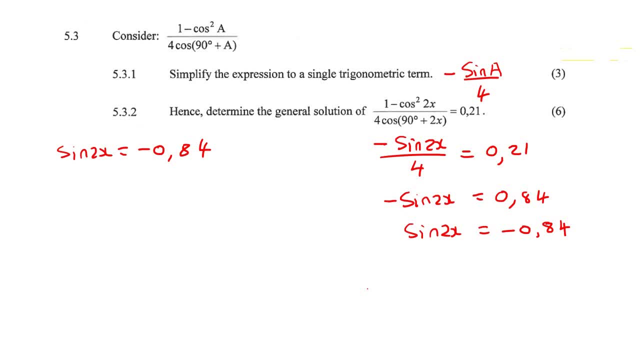 but you don't put the negative on the calculator, guys. So you're just going to say shift. for those of you using a Casio, which is most of you, you're going to say shift, sin of 0.84, just to get our reference angle. 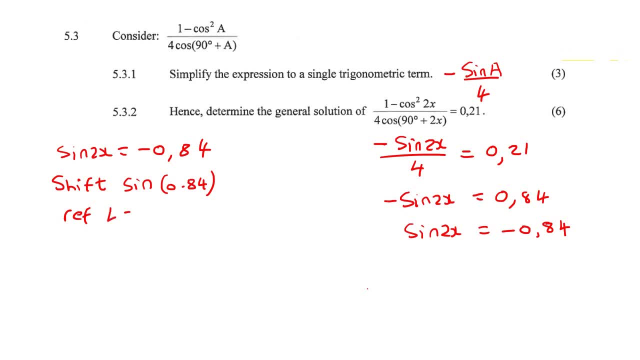 And so the reference angle reference angle will be 57.14.. Now, I'm not going to round off. Okay, I won't round off until the end. So that's that, Now the negative. you might be wondering: okay, well, what does the negative do? 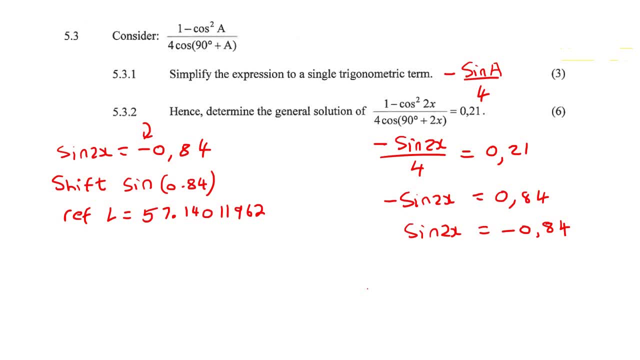 Well, the negative tells us that we are in the quadrants where sin is negative. So, if we think about our cost diagram, where is sin negative? Sin is negative in the third quadrant- This is the third quadrant- and in the fourth quadrant. 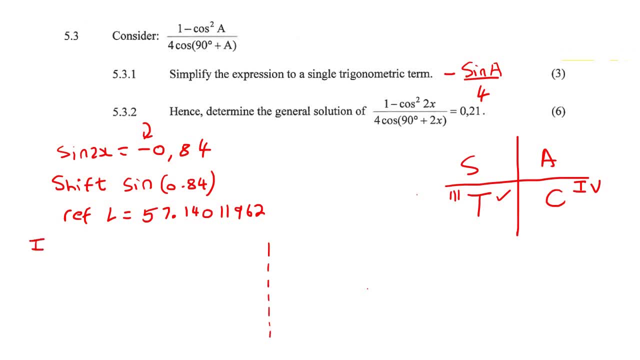 So we are going to go work in the third quadrant, Okay, The fourth quadrant, So in the third, okay. so now what we do is we say, whatever this angle was, that's 2x, So we say 2x equals. 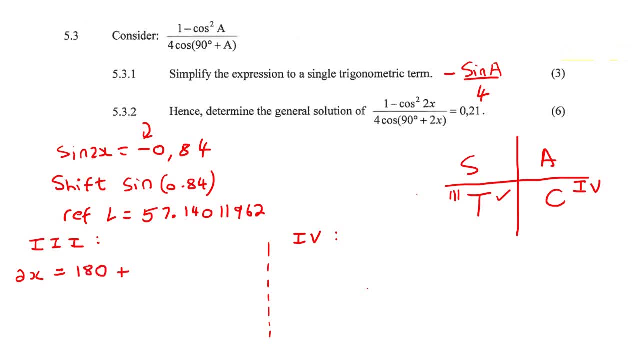 Now in the third quadrant, we always say 180 plus. Okay, I'll carry on with that now I just want to show you guys that it's actually just a pattern. In the fourth quadrant, it's 360 minus. That's what we say. 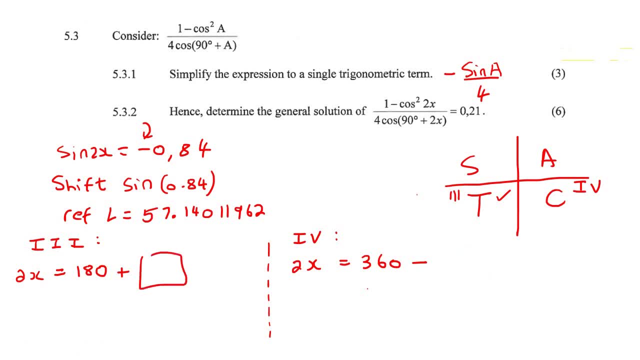 Now, over here we put the reference angle that we calculated, which is the 57.14 value. Okay, and I'm going to put it over here as well. And then, of course, we have to remember that boring old part: plus k, 360, k as an element of z. 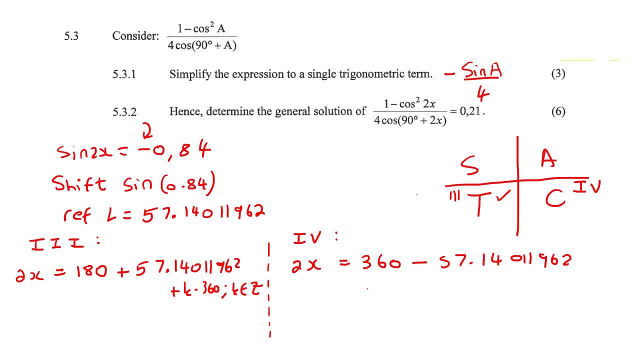 You might use a different letter. You might use the letter n. A lot of schools do that as well. That's absolutely fine. They really don't care about that. in the exam. k as an element of z. Okay, now we just need to go get x alone. 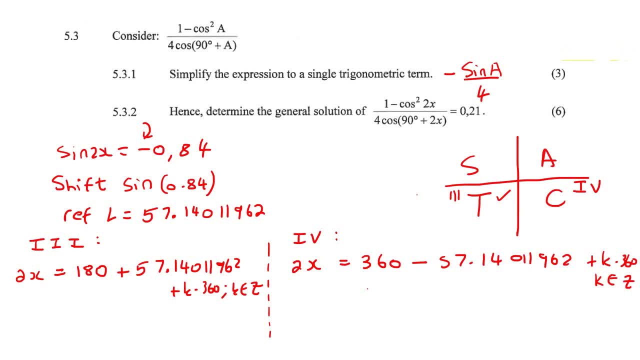 So we're going to get okay, so I'm going to do it all in one step just to save space. But you're going to add these two numbers together, Okay, And then you're also going to have to divide everything, Okay, let me show you that part. 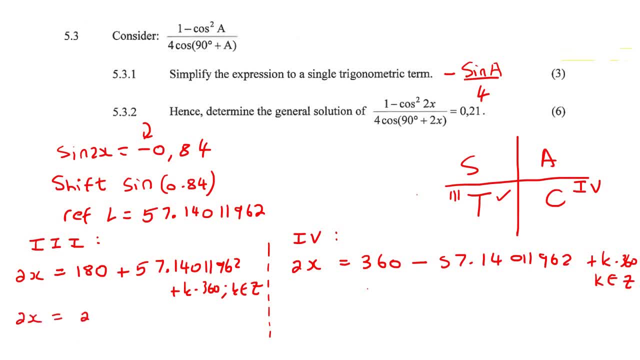 So 2x is going to be equal to 237.1401196, plus k, 360, k as an element of z. Then to get x alone, you're just going to divide everything by two. Okay, so you're just going to divide that one by two. 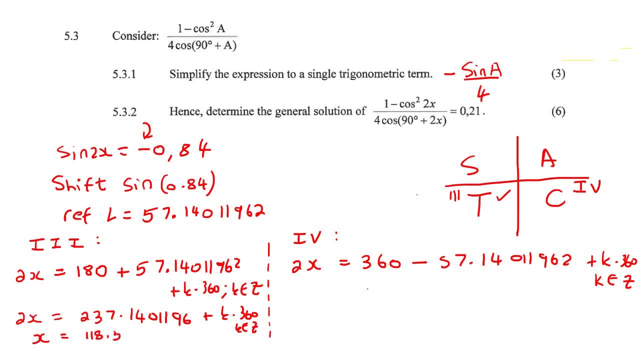 And so you're going to end up getting 118.57 plus k times 180.. So it's important that you also divide this one by two. Okay, So you divide that one by two, And then k is an element of z. 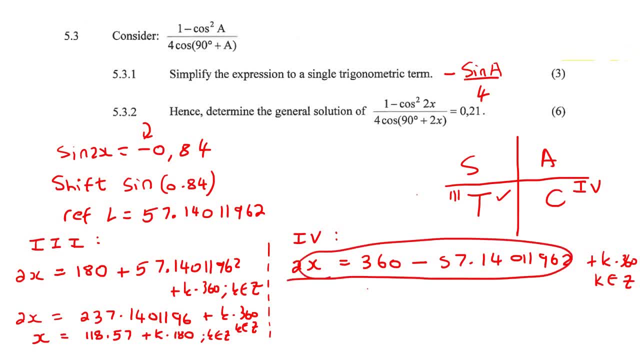 And then we're going to go do the same process for this one over here now, And so if you had to put those two numbers together, you're going to get 302.859.8804, plus k, 360, k as an element of z.